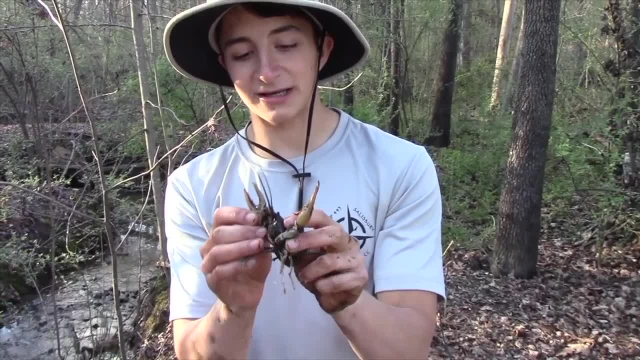 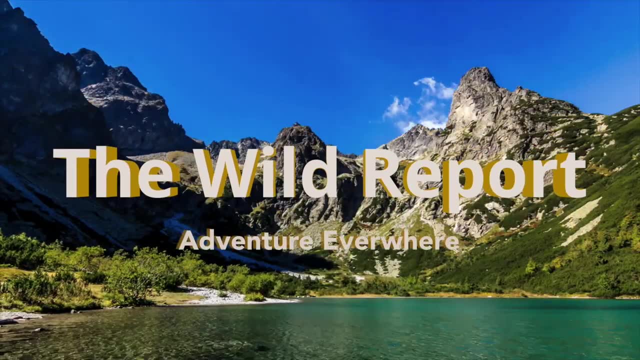 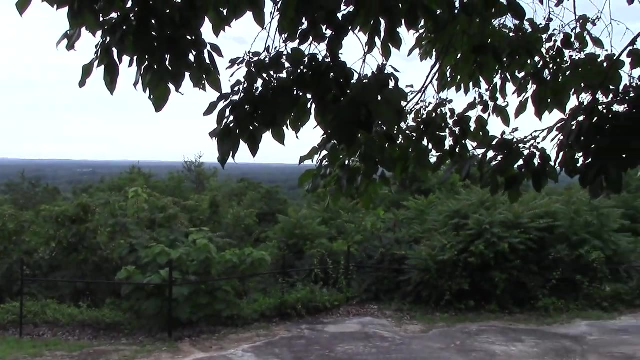 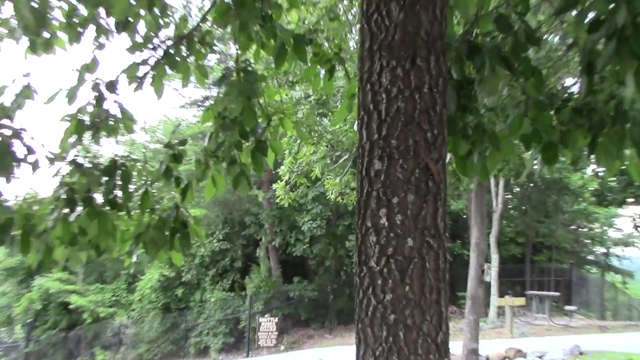 Lizards are some of the most common reptiles around, able to be found in a variety of habitats, from deep in the wilderness to right outside your door. In this episode, I'll be catching some lizards that you might see around your house and explaining why they should be left. 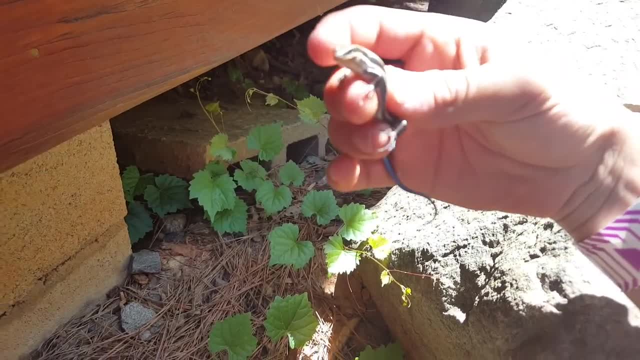 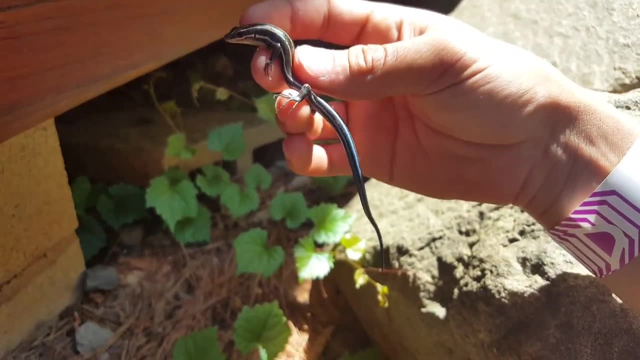 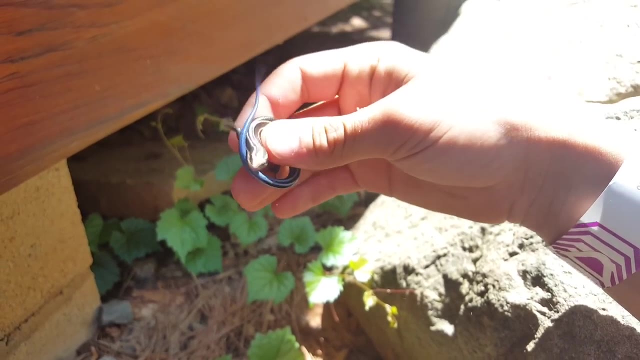 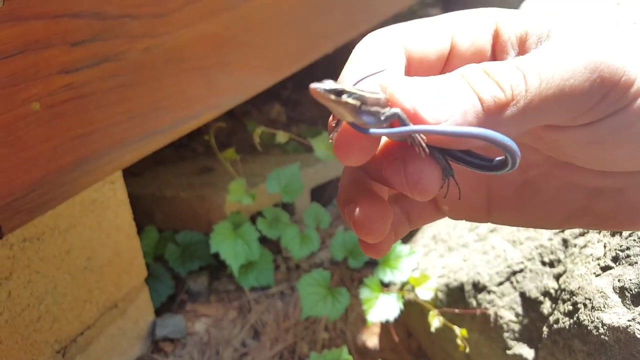 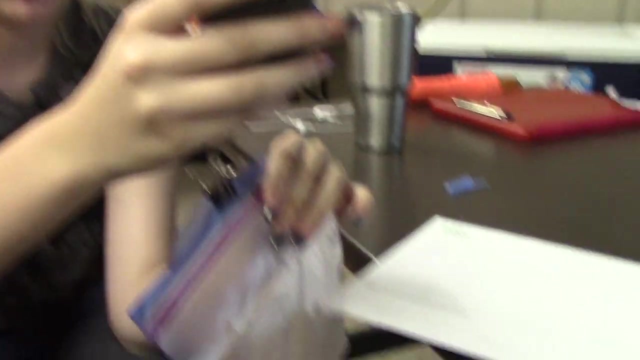 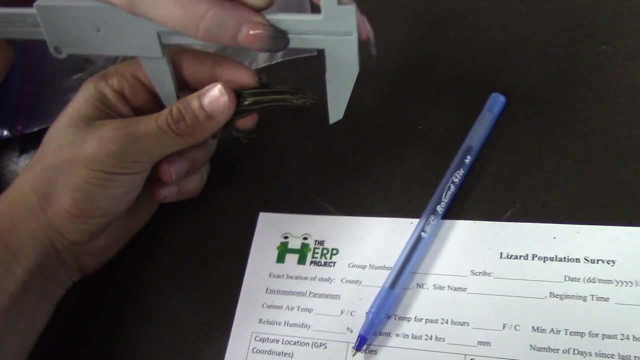 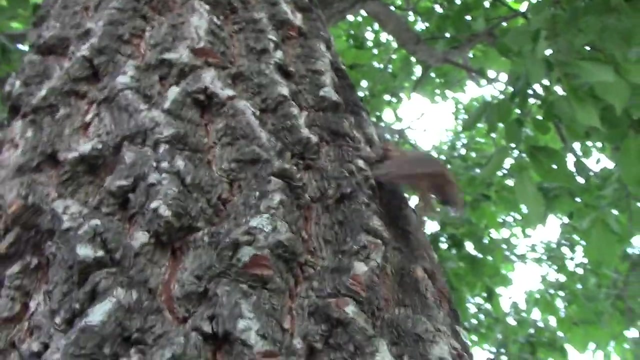 alone instead of removed. Now, after catching those skinks, I actually had the chance to collect some data on them for a really cool citizen science initiative called the Hurt Project, which I will cover in a later video, But today I was on the hunt for the very quick and agile eastern 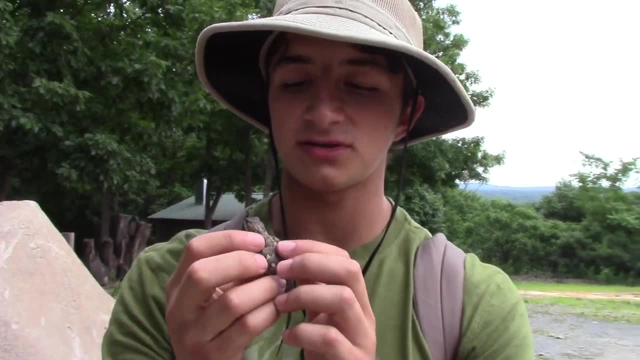 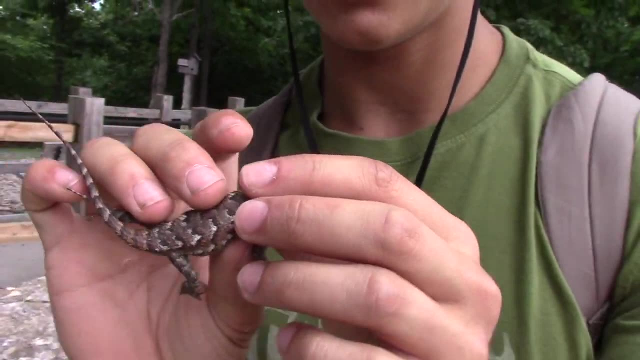 fence lizard. Now, fence lizards have rougher scales than most other species we have around here. Their scales are keeled, so they actually come to a little ridge in the middle, and what that does is, let's say, I was a predator and I grabbed this. Well, when I put my finger in, 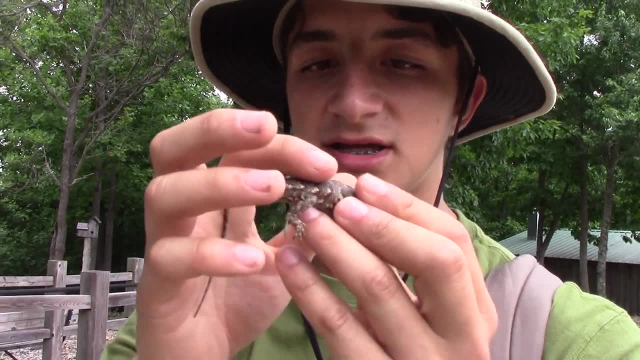 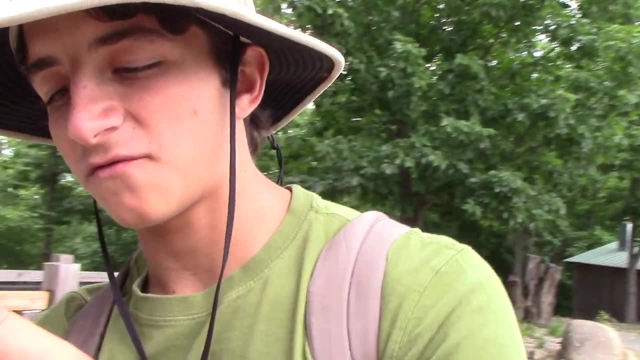 my mouth. if I'm going this way, his scales are going to stick into me, into the roof of my mouth if I'm a predator, which is really uncomfortable, obviously. Now, these also have a very different body shape than things like five-lined skinks or six-lined race runners. 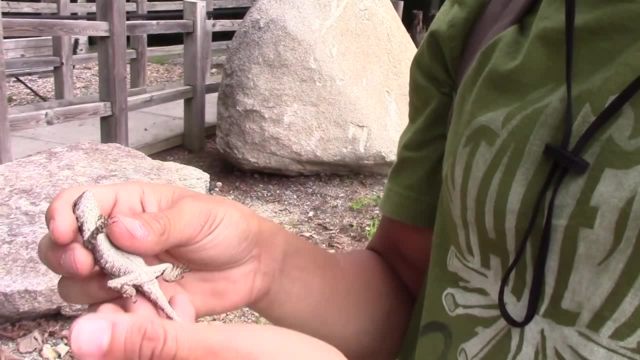 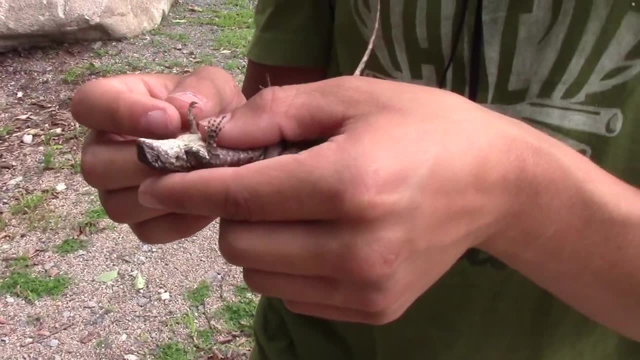 we have around here. They're definitely built very differently. They're a little bit stockier Kind of, looks like an iguana Kind of In a way, And they have these really broad hands with these claws made for gripping things. So these 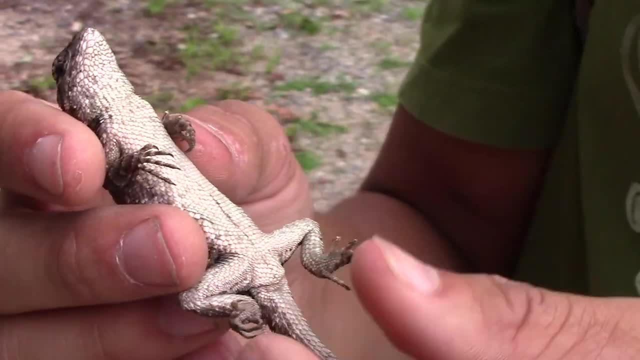 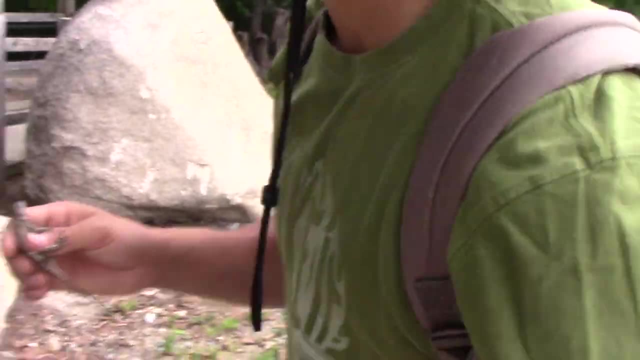 can run on just about everything. They're really, really cool. Cool lizards- And this is a really pretty one as well- Very, very cool lizards. I'll show you just how fast these guys are from here. While that was a neat-looking individual, I knew that we could find a more impressive. 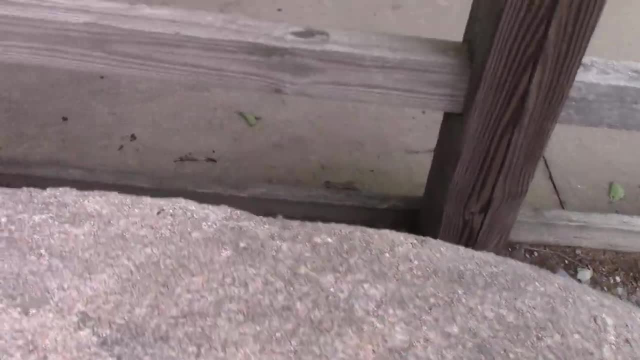 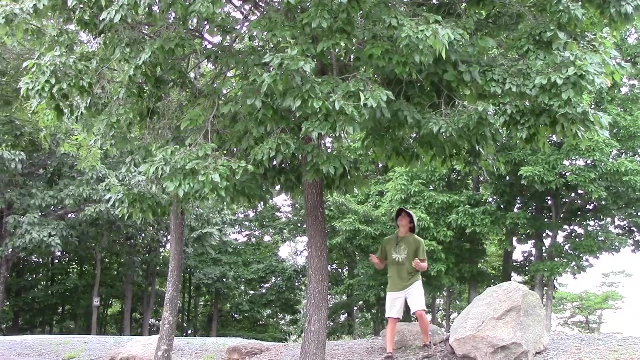 specimen, and so I began searching for a male. All right, guys, We have a fence lizard up in this tree. Now he's probably about 15 feet up there, but I've got to catch him, So I'm just going to get the tree somehow. 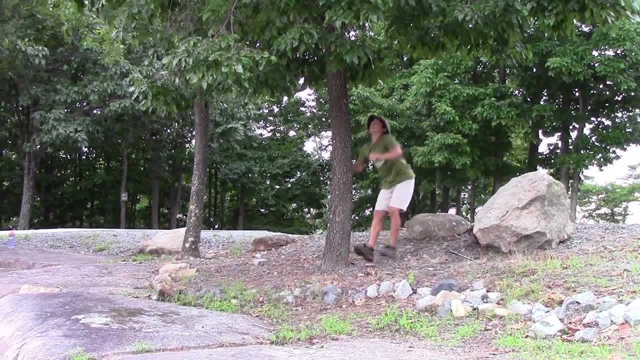 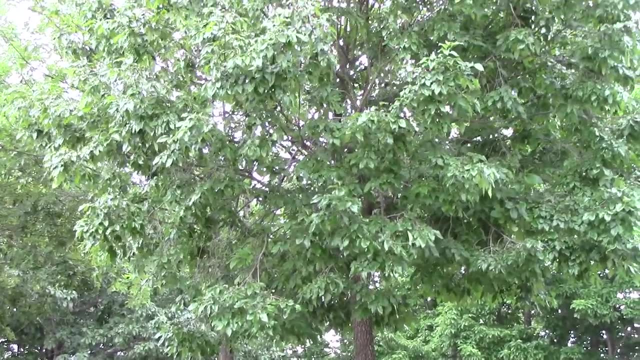 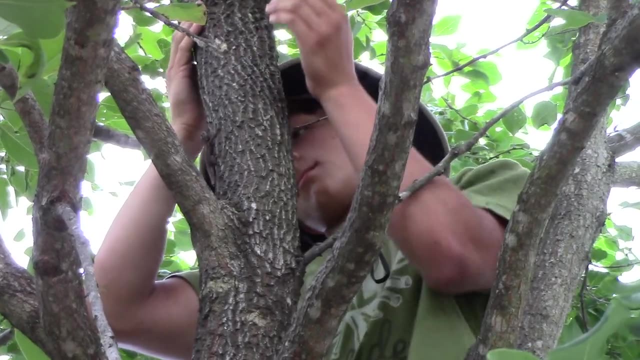 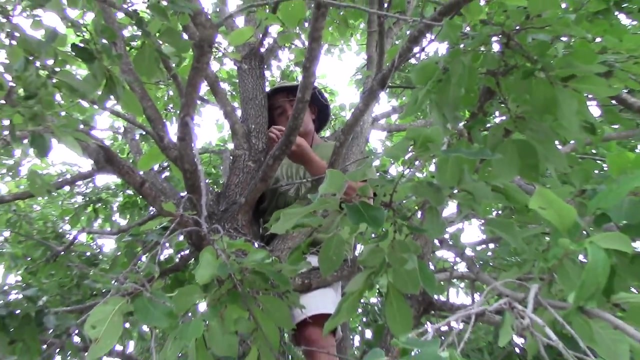 We're going to have to go make an insane creature grab here. Oh, I see him. Yeah, he is there. Yeah, he's right there, Got him. Ooh, that's a male, That's a really pretty male. Is he actually missing part of his tail? 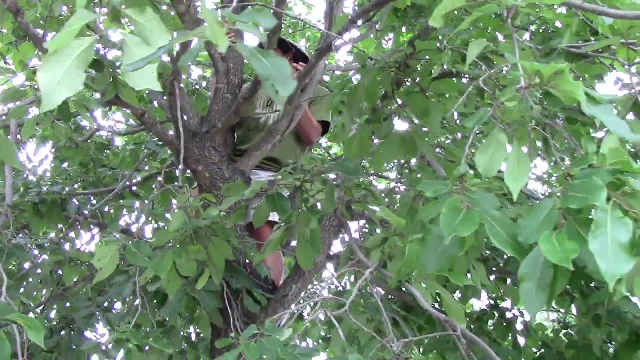 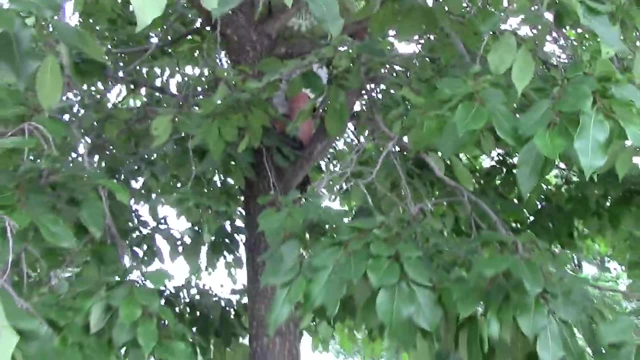 Oh wow, He's gorgeous. We're going to bring him down, guys. How high up was he? Like 15 to 20 feet. You're about 15 feet up right now. That's what you've got to do for a creature catcher sometimes. 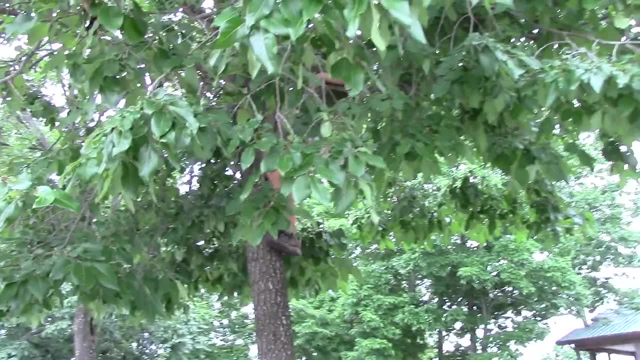 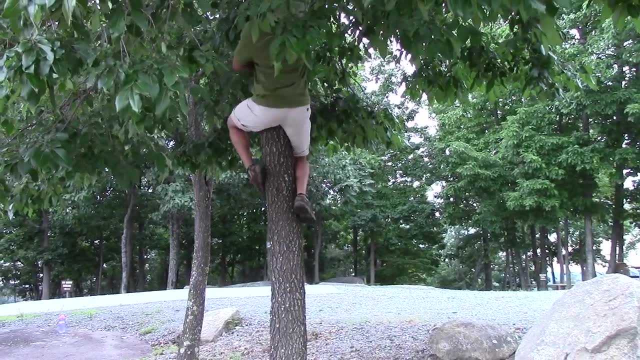 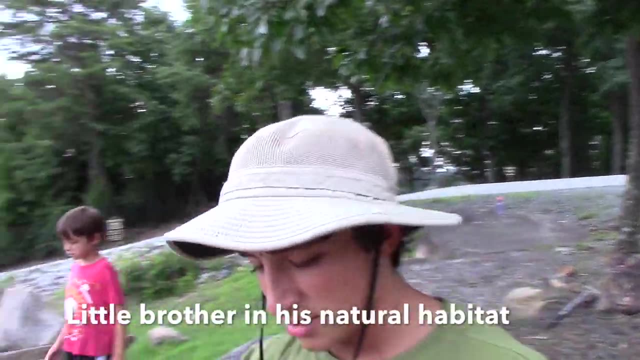 All right, now we've got a lizard on one hand And you're jumping down with the other hand. All right, So that's another fence lizard, but this is a male. You know how you tell. Look at that. Look how pretty that is. 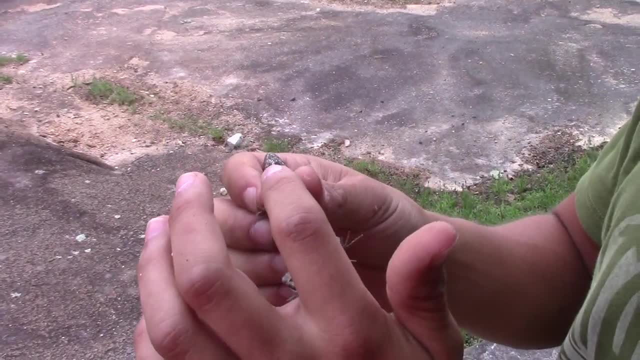 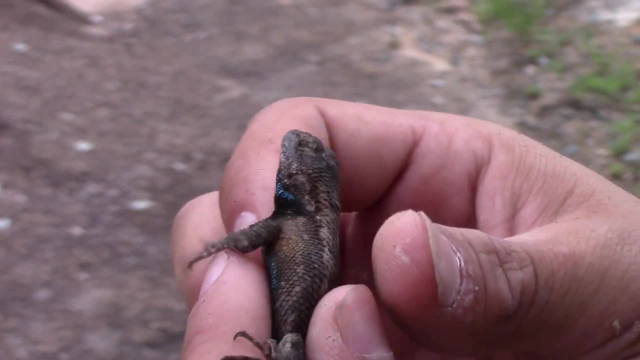 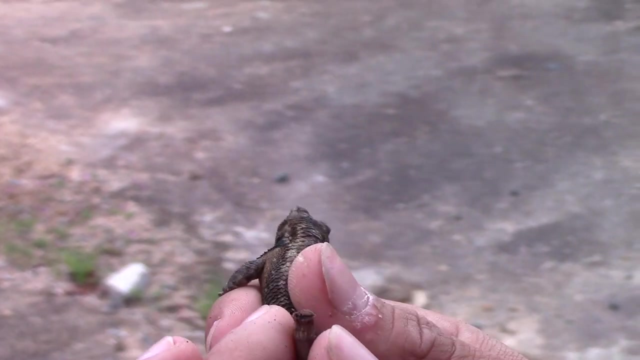 There's the gorgeous iridescent blue teal color there, there and there The males have that color to attract mates. Now this one actually has detached part of its tail at some point in time as a defense from predators, which is another thing these lizards will do, And luckily it wasn't a response. 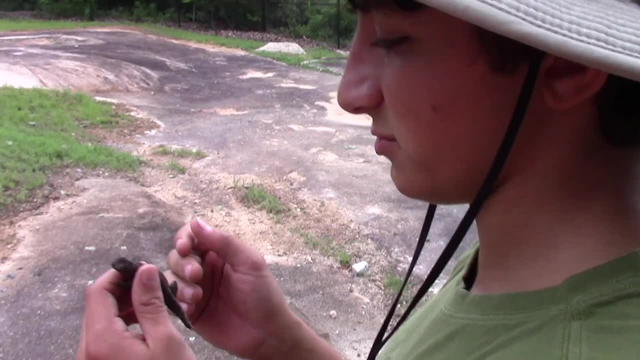 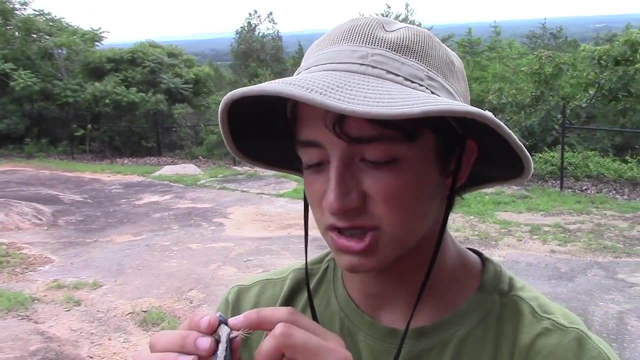 to me He'd already lost his tail. Maybe why I was able to catch him is because he's a little bit slower from that, a little less balance in that tree. But you see the males, like the last lizard, they have that really gorgeous accent right there. I love that there's. 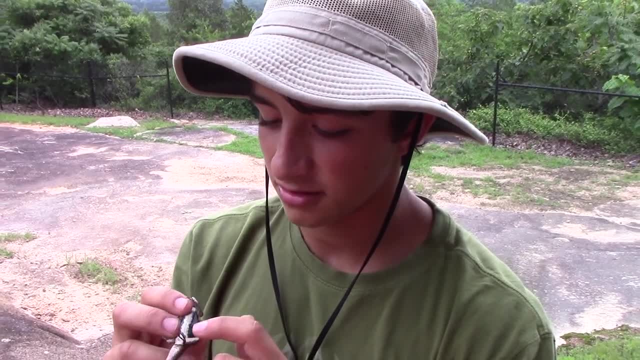 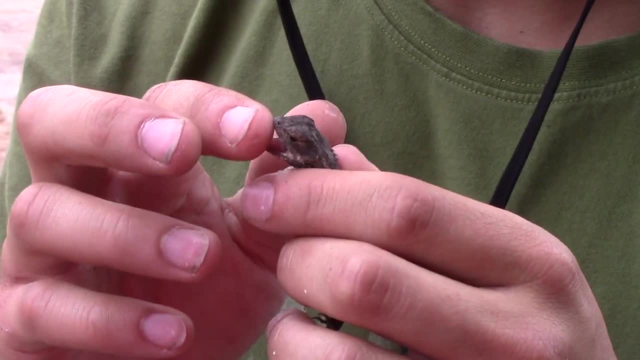 no other lizards in the state, I think, that have that really iridescent blue color on their scales, like that, really, really cool. I actually take a picture of him now. he's not very happy right now. these things will bite you. they don't really enjoy being handled, but they're really cool. 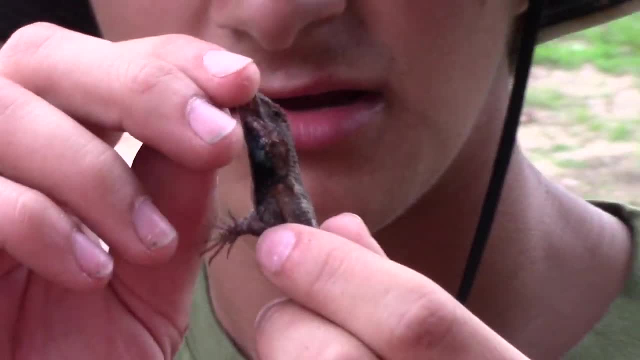 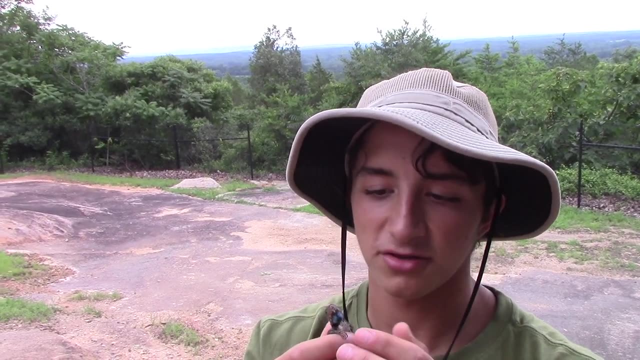 lizards. they're really gorgeous. I can take some pictures of that blue. we'll get him right back in his tree now also fence lizards. they're insectivorous, just like all the others we've talked about today, and they are extremely, extremely quick, these claws, just let them. 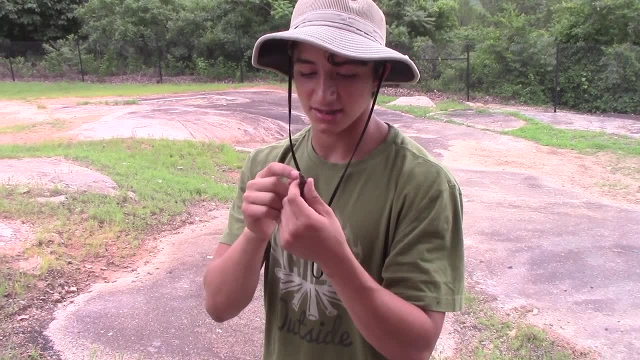 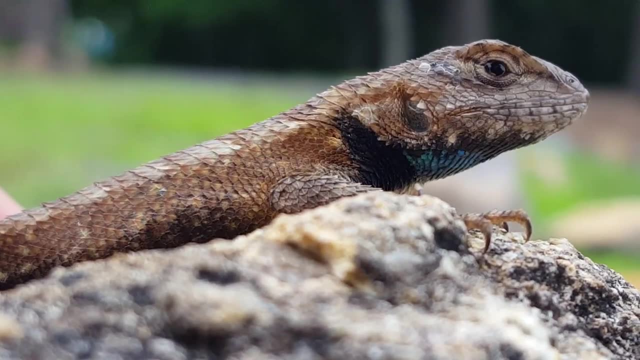 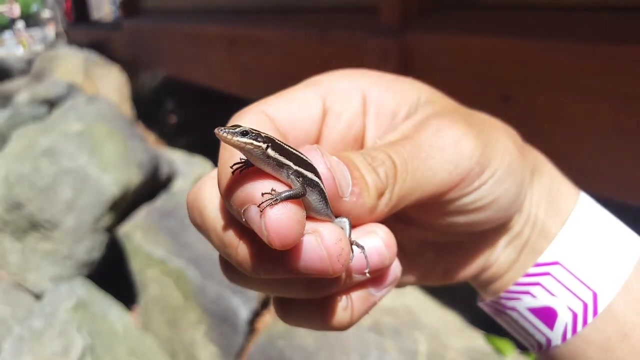 scurry up any rock, tree, wood, anything, to catch insects. it's really cool. many people who have a population of lizards living in or around their house choose to exterminate them, either using a professional service or glue traps to catch and eradicate the animals. however, if you do,